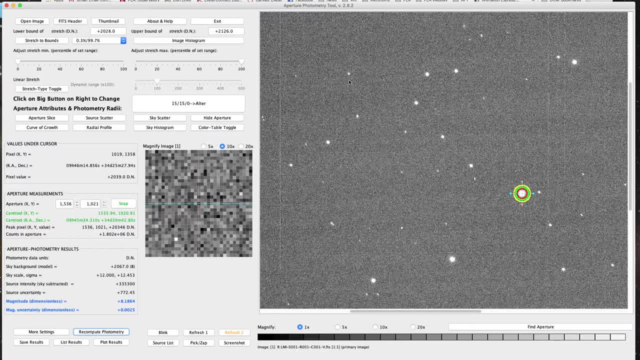 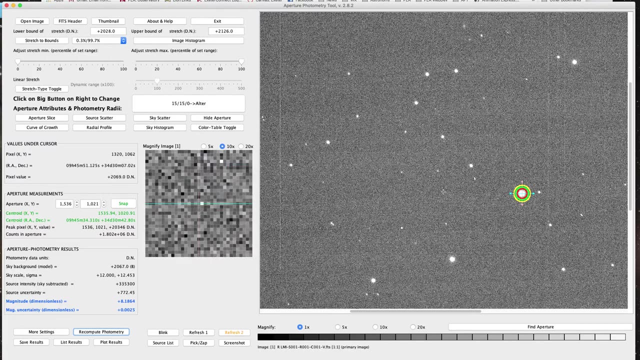 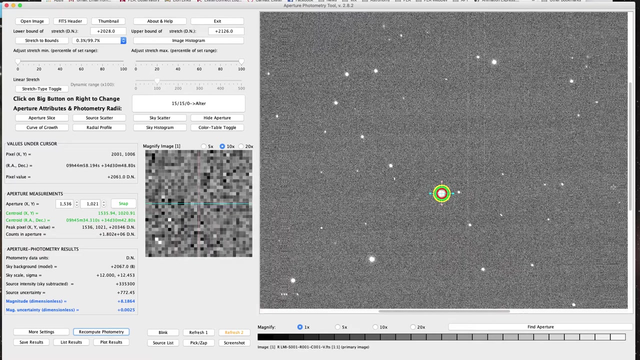 stars in question versus your comparison stars and then trying to fit a zero point to your photometry in order to get a correct magnitude readout from the APT software. So I have opened here an image of a fairly well-known variable star called R leo minoris. 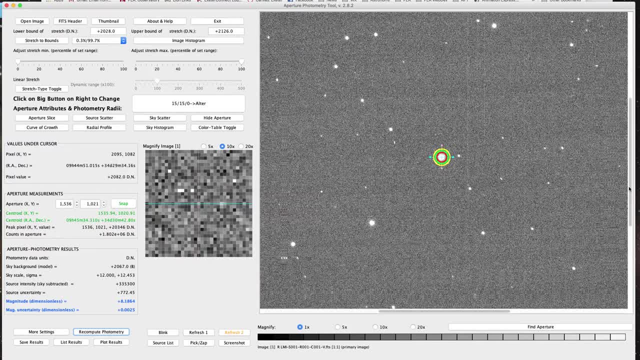 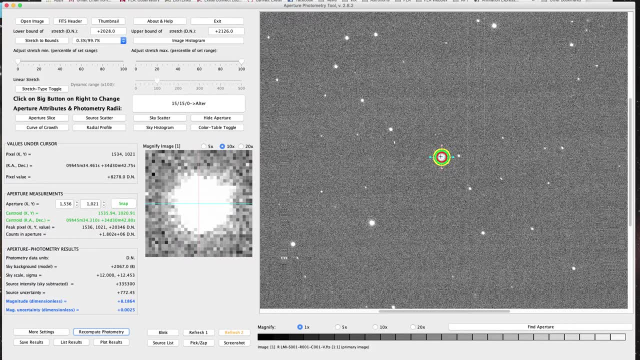 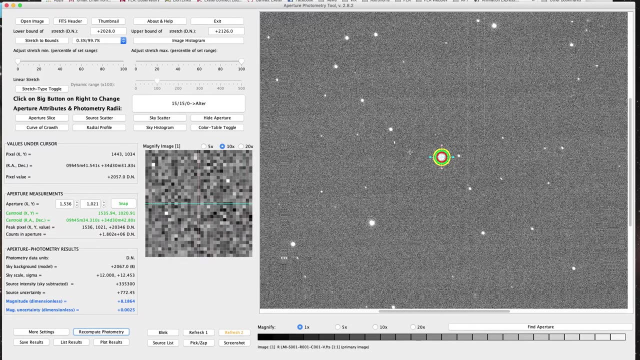 and it is located right there in this aperture here And the apertures have already been set. I'm not going to talk about full width, half maximums and how to set the aperture radii and whatnot. That is also discussed in the prior video that you've seen. 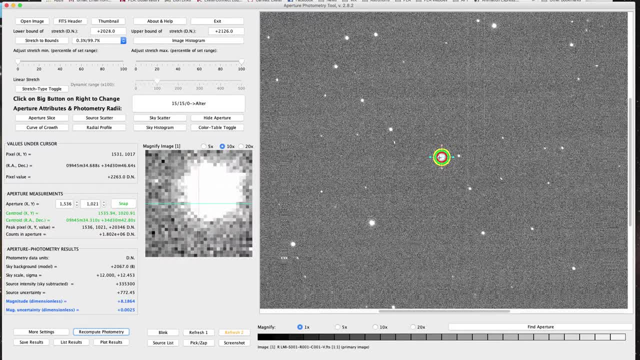 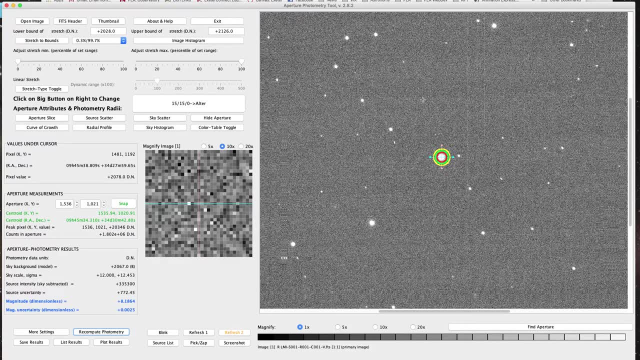 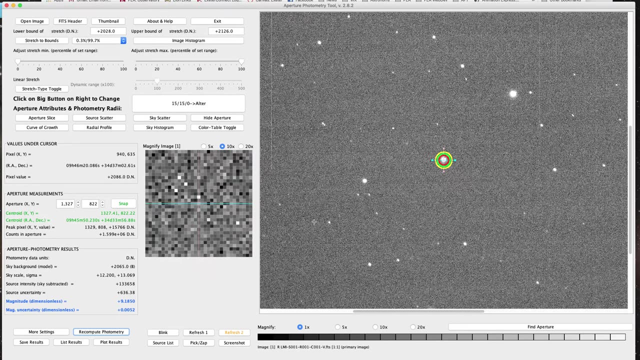 You should watch. So we've got our star here and what we want to do is figure out what this star's magnitude is relative to a comparison star or two. And to do that one can't just click on a star in the software and then down here on. 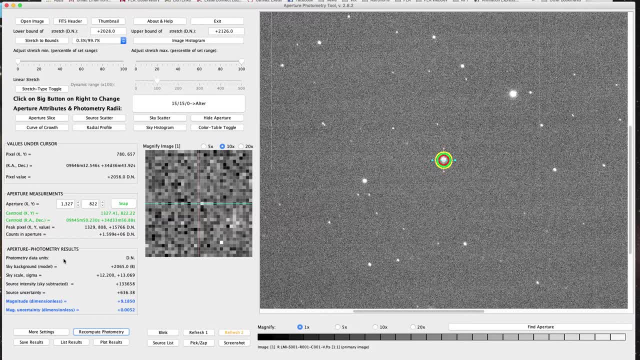 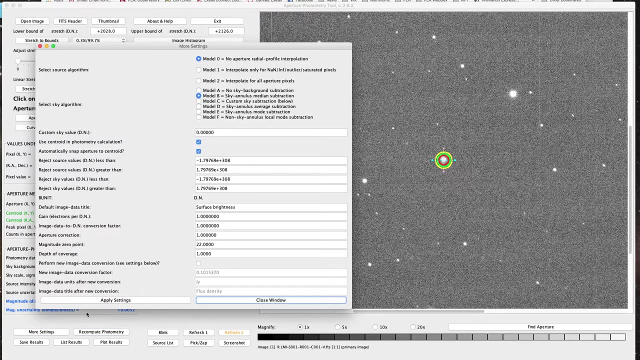 the lower left, see where it says Aperture Photometry Results. One can't just hope that the magnitude here, which is 9.1850, is correct, Because it probably isn't, And the key to that is located under this More Settings button here down at the bottom. 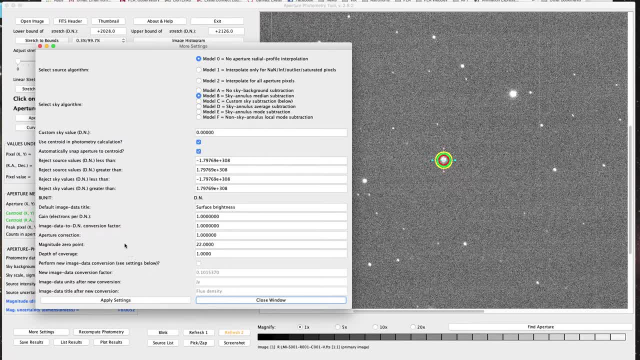 When you look inside the More Settings button, a couple things that are really important is that you really want to have your select sky algorithm set to Model B, which sets a sky annulus median subtraction from the region where the star is actually located inside the annulus. 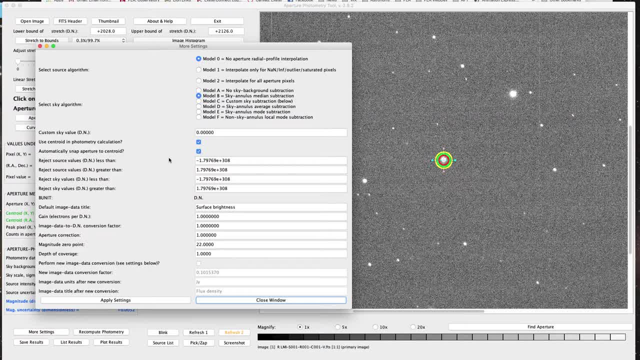 You could also use average as you see fit, depending on the situation. So you could also use average as you see fit. depending on the situation, You could also use average as you see fit. depending on the situation, You can also use average as you see fit, depending on the situation. 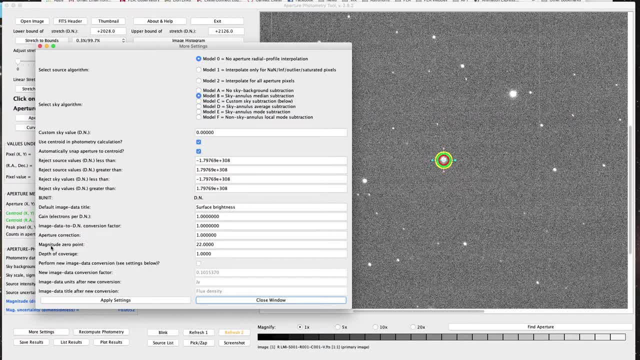 You could also use average as you see fit, depending on the situation. So you could use average for fixation, joke about it, even if you don't know the type of work that you're doing. But, more importantly, setting this to magnitude zero point is really important. 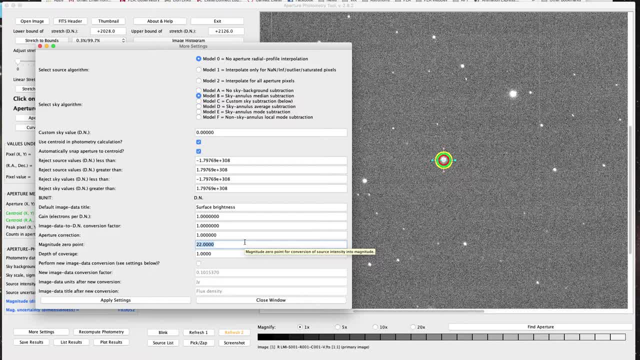 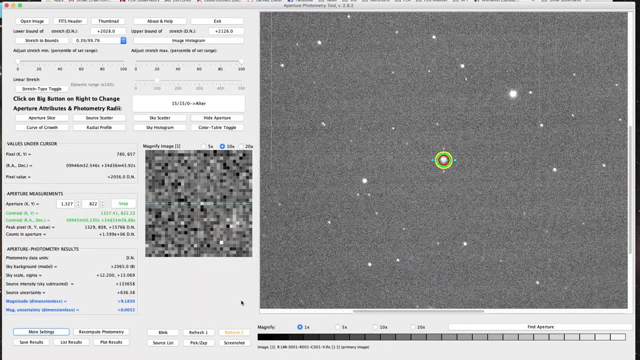 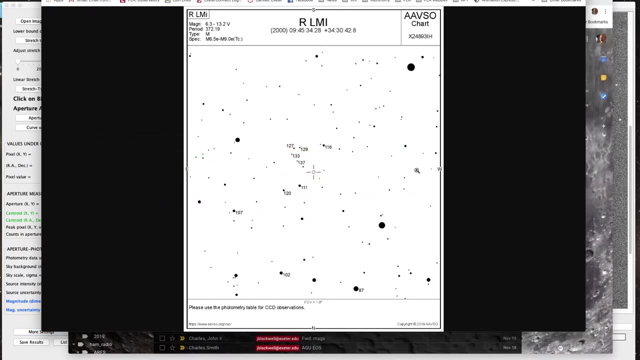 This value of 22.0000 is nonsense. I just stuck that in there. So how do we find out what the magnitude two zero point is? Let's close this window and then let's take a look at our star field. Then let's go over here and look at the AAVSO chart, the finder chart for our LMI. 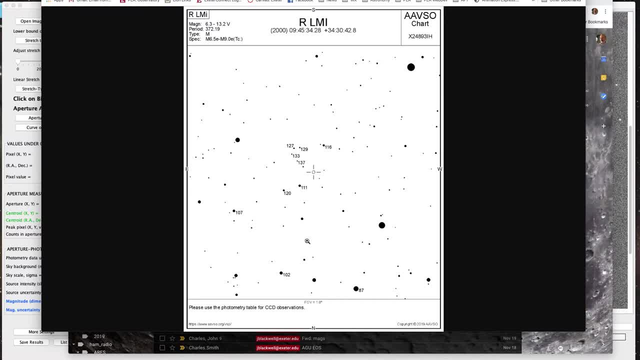 In LEOminer and you can see that we've got a number of really good comparison stars here to choose from. I'm going to point out the 12.7 and the 12.9 here. Let's look at 12.7.. 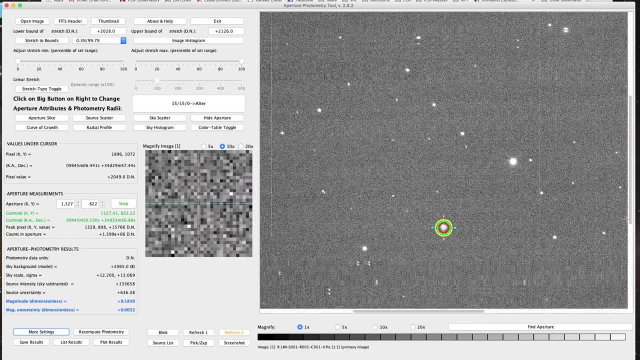 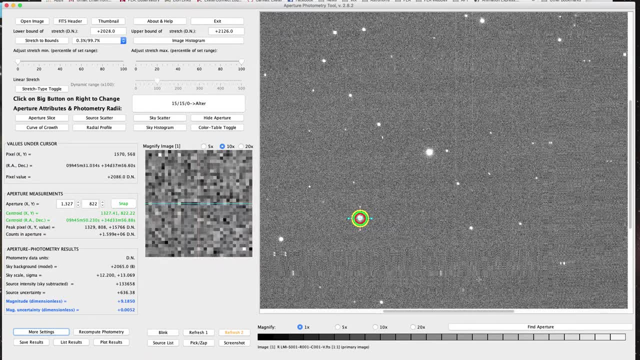 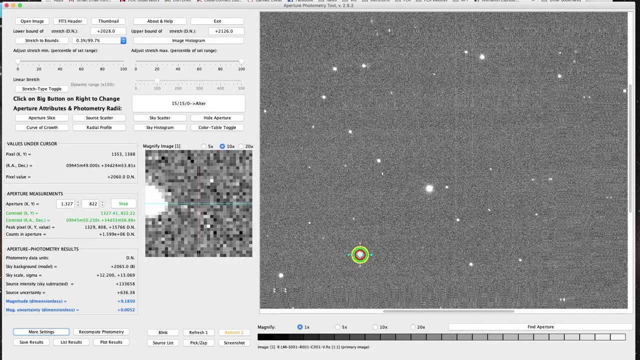 That star is. let's see if we can locate it quickly and get RLEOMiner up in view. here It's RLEOMI, and then you've got these two stars up here. the left one and the right one are the 12.7 and the 12.9.. 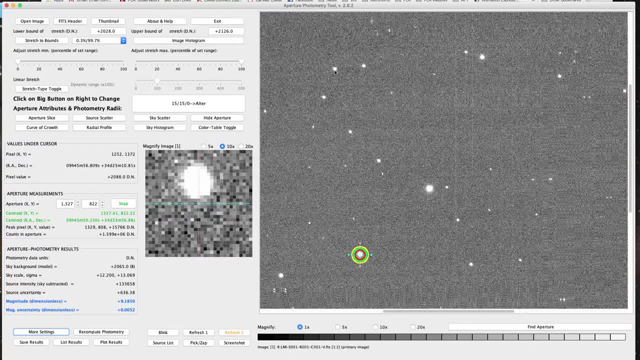 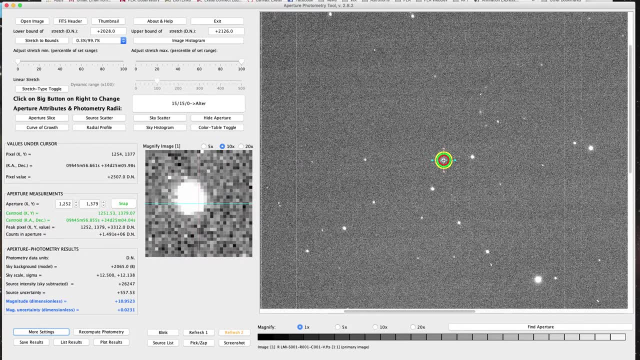 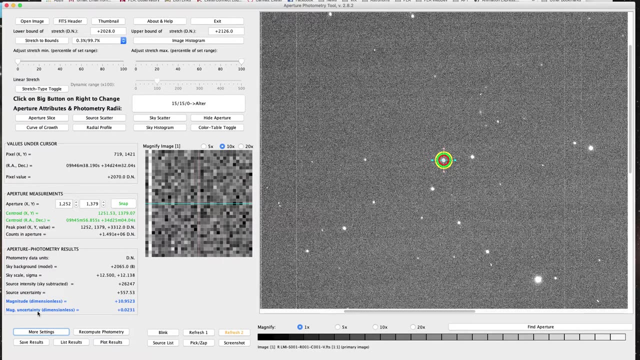 So here's the 12.7,, here's the 12.9.. If I select the 12.7 star and get it nicely centered in terms of the annulus, get it clicked on, there we go. the software will report a source intensity with sky subtraction. 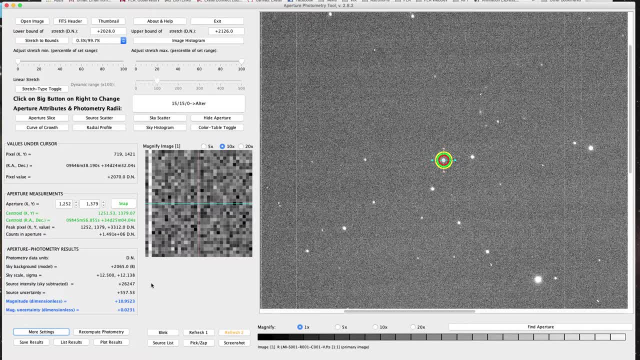 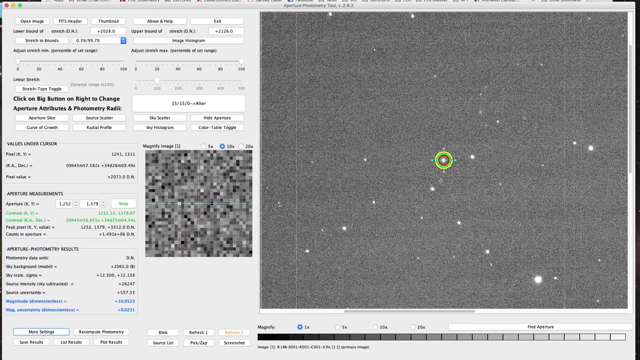 Subtracted of 26247.. So that's the pixel count, the intensity of the star's light, with the background sky's light subtracted from it. We can use this value, since we know what the magnitude of the star is, in our filter. 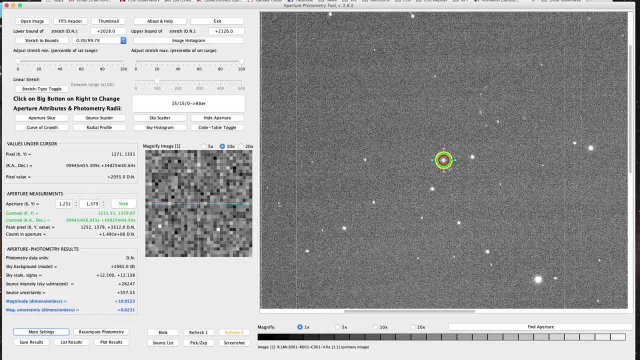 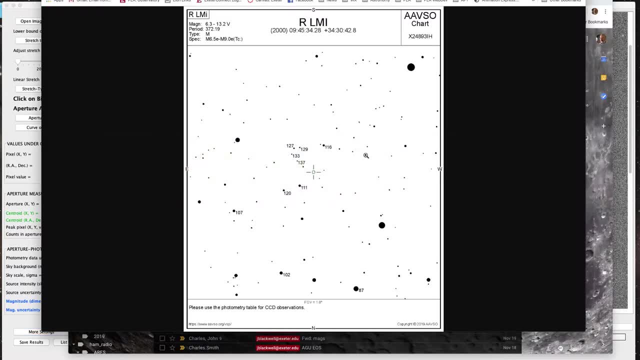 By the way, this is a V Johnson-Cousins photometric filter that we've used here for V visual or green, as the case may be- And we go back to the AAVSO website and we're like: ah 12.7, what is its accurate magnitude? 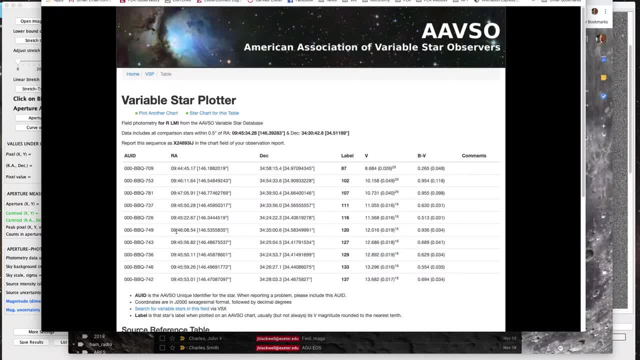 And we can go look at the photometry table for that. And so for the 12.7 star here we have a V magnitude of 12.686. And we can use that. So 12.686 is the known magnitude. 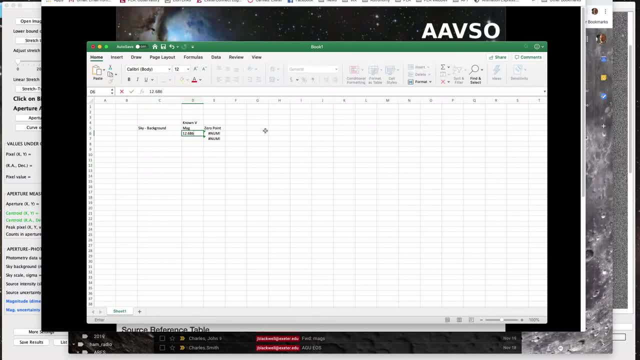 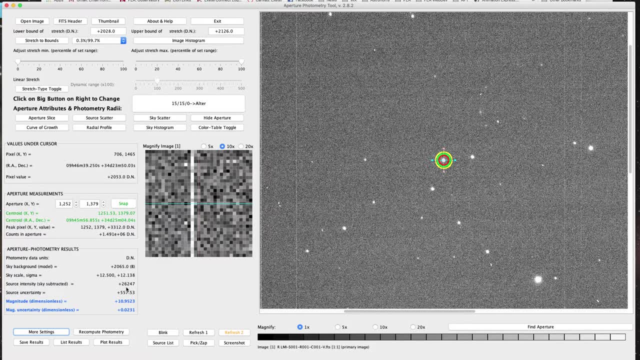 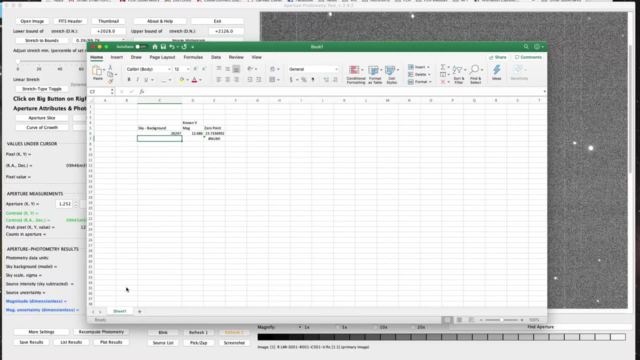 So 12.686 is the known magnitude. The SkyMize background count in our image is down here at 26247, so I'm going to enter that 26247 and I've created this little spreadsheet in Excel that will automatically calculate the. 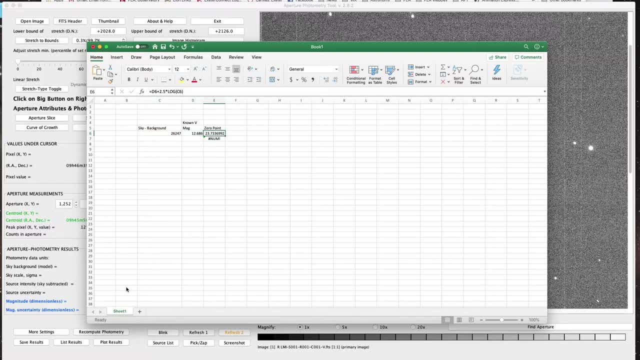 zero point. the zero point is simply the known magnitude of the star plus the instrumental magnitude of the star in your image. so this is going to equal the known magnitude, 12.686, plus 2.5 times the log to the base 10 of the sky minus background value, or the instrumental magnitude, which is 26247. 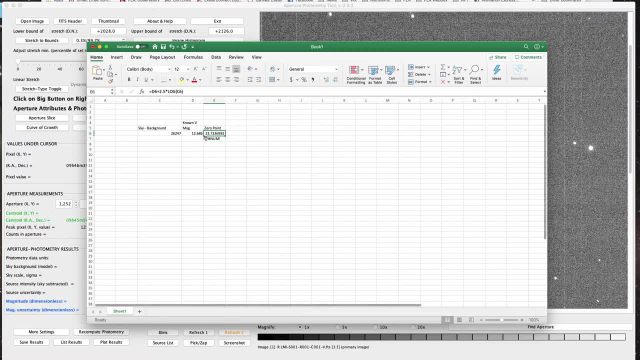 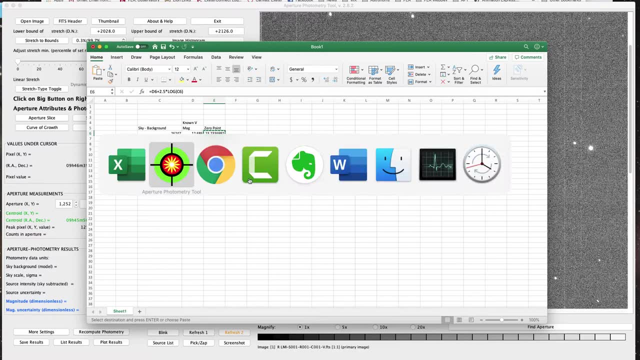 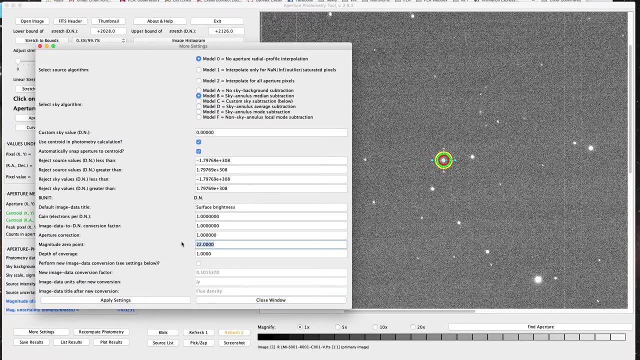 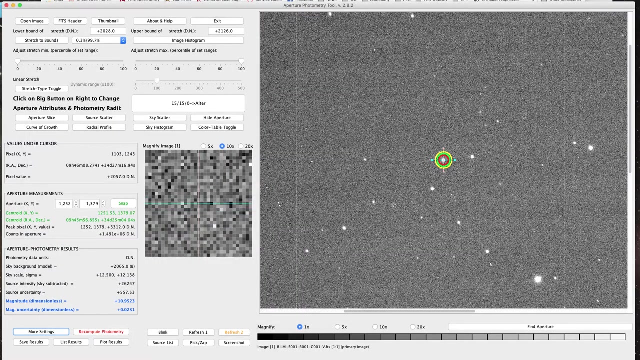 and you end up with 23.7336992 as your zero point. so if I copy that and then go back into APT, go to the more settings, go to the magnitude zero point, go in and say: apply settings and close window, you'll now see that if we click on the star, 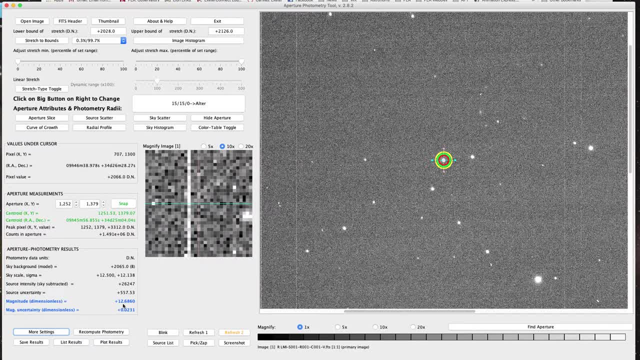 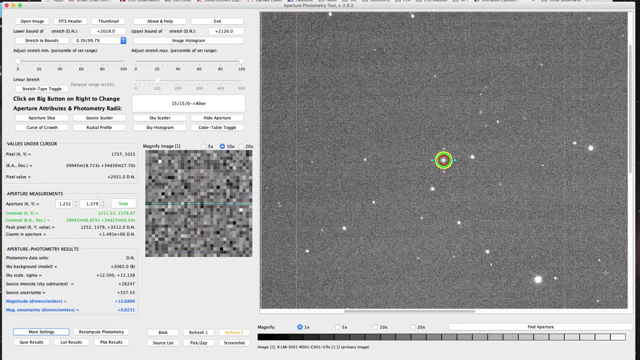 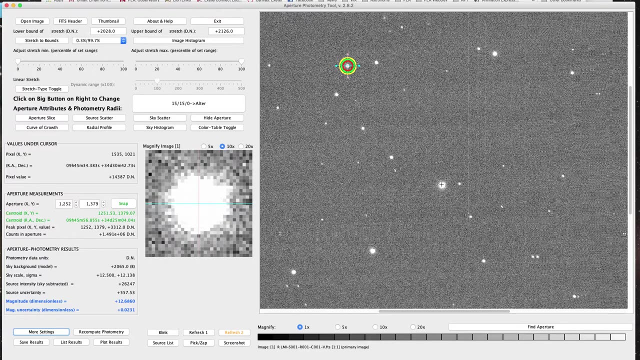 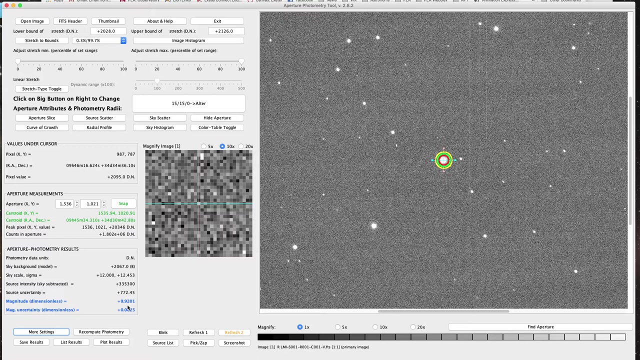 down here that you get a magnitude of 12.686. lo and behold the correct value. not bad. now, if you go down here and you click on our LMI, it will report a magnitude of 9.686992. that's basically how it's done. 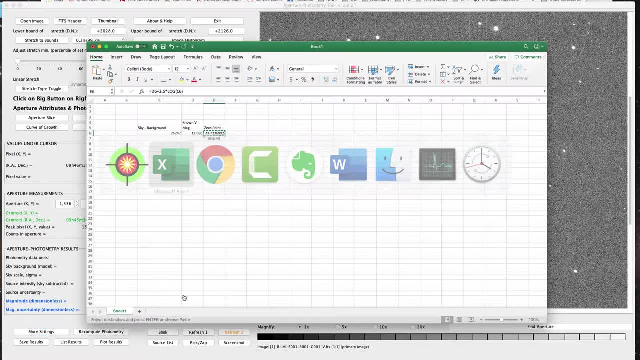 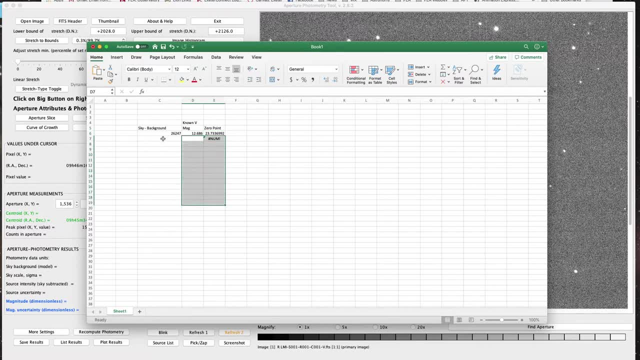 nice and simple. if you are looking for more precise values, you could do more of these known magnitudes versus sky minus background values and collect more zero points across the image and then perhaps average them together and get an average zero point for the entire image. there are a lot of ways of. 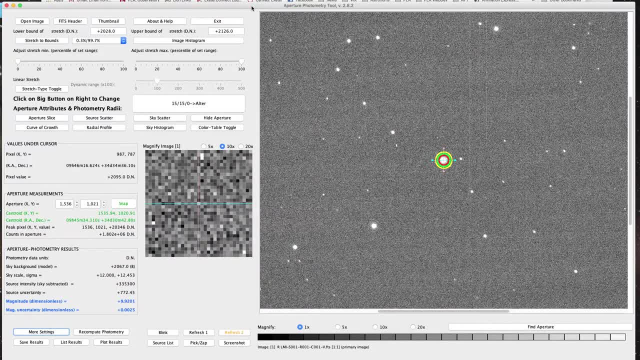 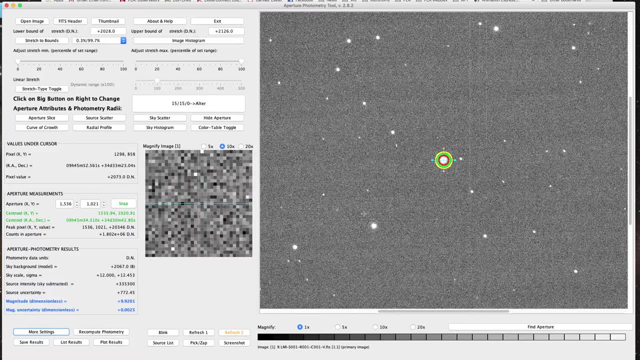 doing this. there certainly are a lot of ways of doing this, but that is a really quick way of getting a zero point out of an image for yourself. now, things to be wary of. if you look in this image, you'll see a couple of columns that are bad you want to avoid. 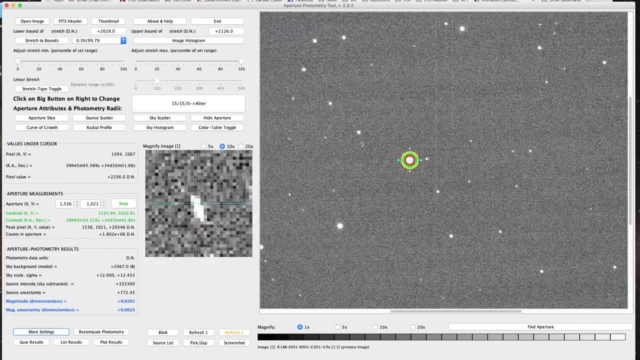 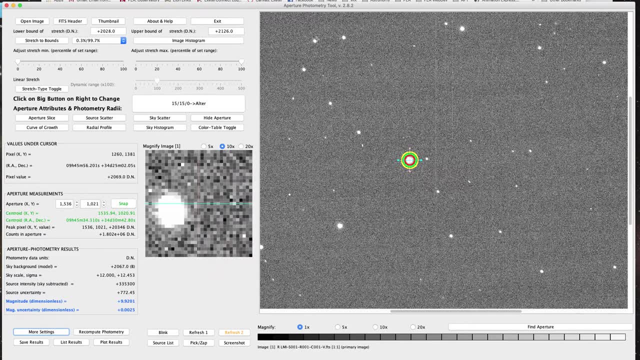 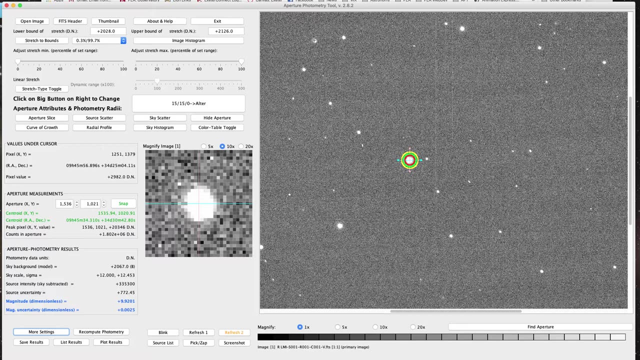 standard stars with bad columns or perhaps some hotter pixels than usual because of a cosmic ray strike. you want to make sure that your stars are not clipped off at the top and, well you know, blooming, for example, If your intensity maximum for your CCD is 655, 35, you don't want to be peeking out up anywhere in that non-linear range. 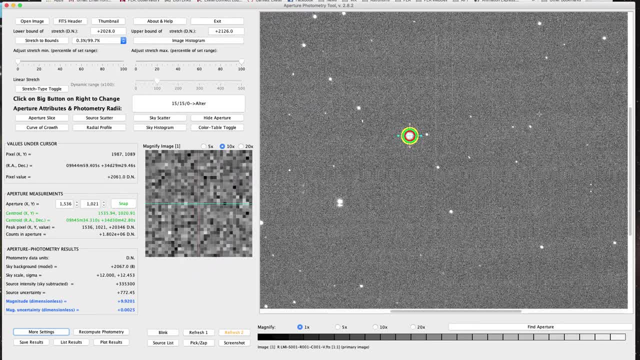 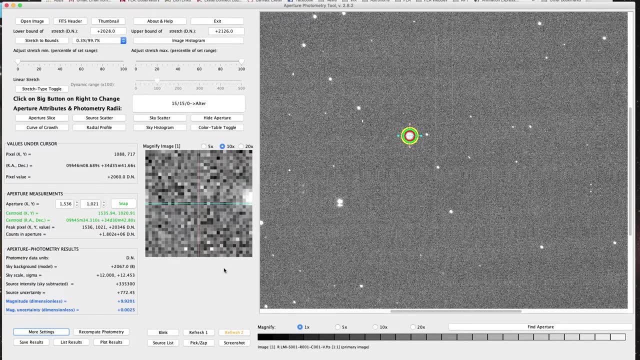 for the sensitivity of your chip. You also don't want to be working in crowded star fields, that type of thing. So there's a really cool thing you can do. And, of course, once you've done this, you could also go through and use the source list tool and it will go and measure all the 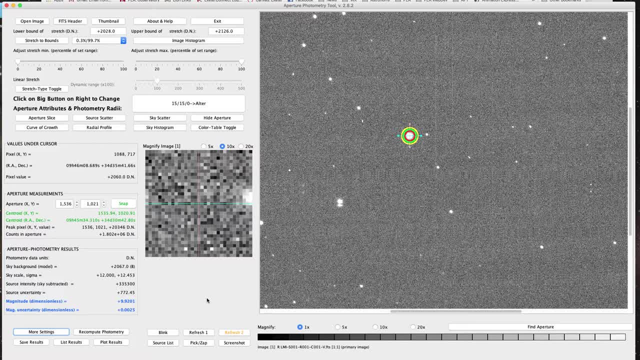 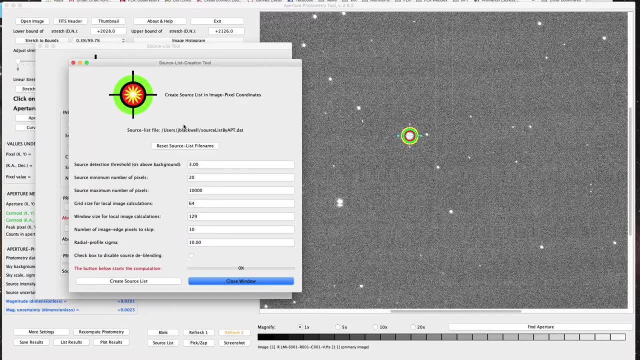 magnitudes for all the stars in the entire image, And that's kind of cool for things like open clusters and whatnot. Kind of a neat thing. If you go in here, we're going to create a new source list. We'll reset the file name. Now we'll just use the file name it has up here. Go up here and 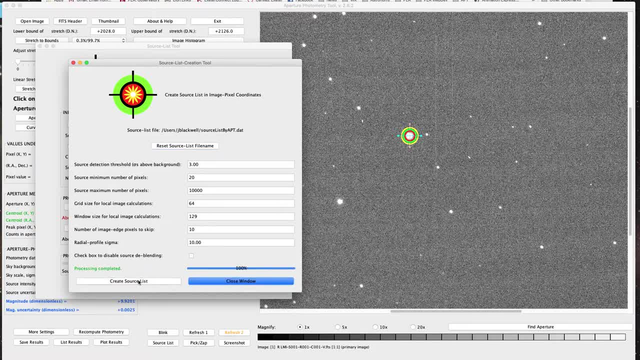 say, yeah, that's really neat. We'll create the source list. It's going to find all the magnitudes for all the stars in the entire image, And that's kind of cool for things like all the stars in the image and life is great. We'll close the window And then we're going to 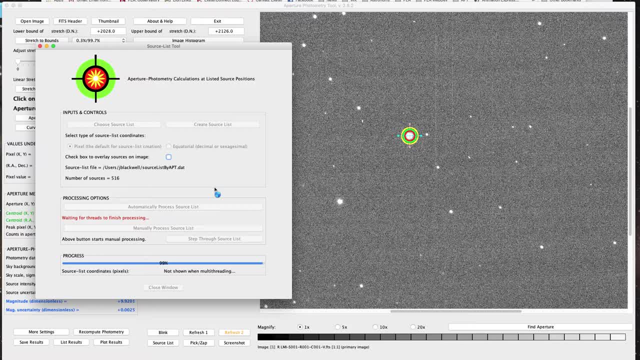 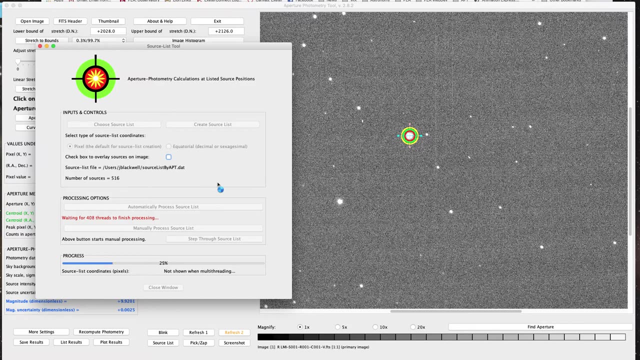 say: you know what, let's process the source list And it's going to do photometry and all of them based on our one star here, our one reference star. Now, that's kind of risky perhaps, but it gives you a quick idea of the power of ABT software If you are measuring an open cluster. 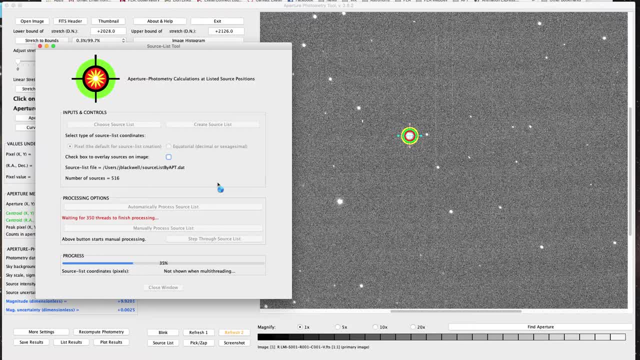 and you're not going to want to sit there and click on several thousand stars for the rest of your afternoon and then try to remember which ones you clicked on in what order. this software will create the source list for you. put them in the correct order. allow you to save off that. 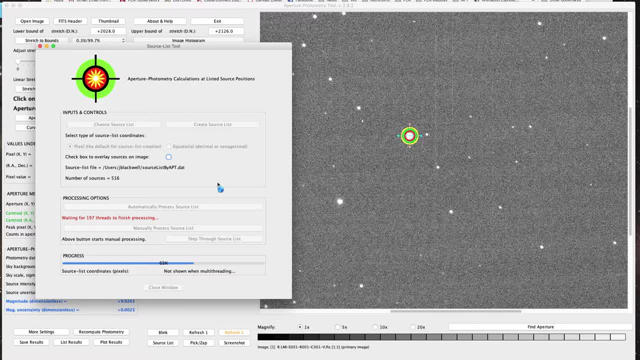 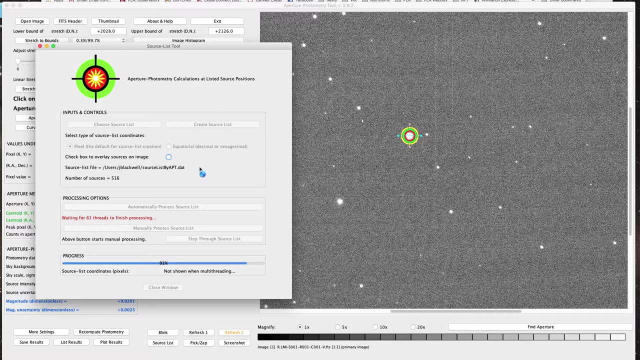 source list and then allow you to operate that source list in several different images of, say, B, V and I filters, which allows you to do some really cool color magnitude diagrams for open clusters. And then you can use spectroscopic parallax to figure out the distance to the. 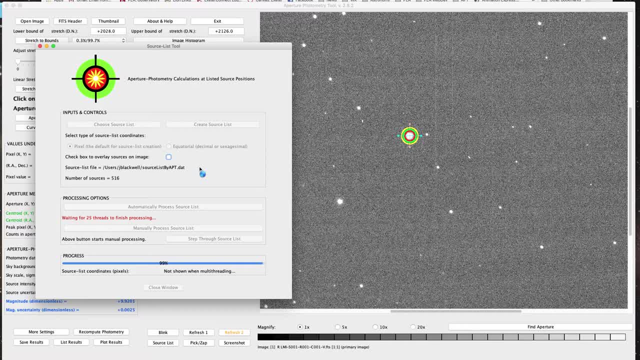 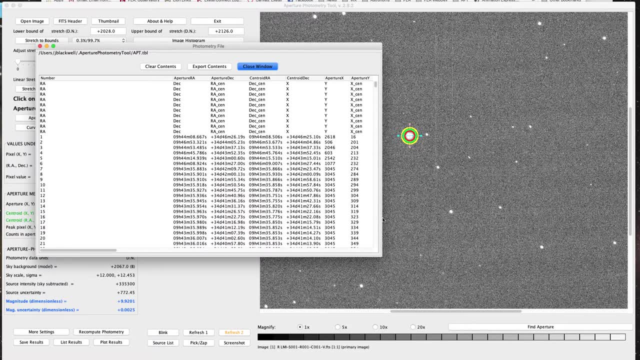 cluster And then the age of the source list, And then you can do some really cool color magnitude diagrams for the rest of the cluster and things like that. So very handy. So once you've got that, you can list your results. You can see all sorts of beautiful stuff happening here in. 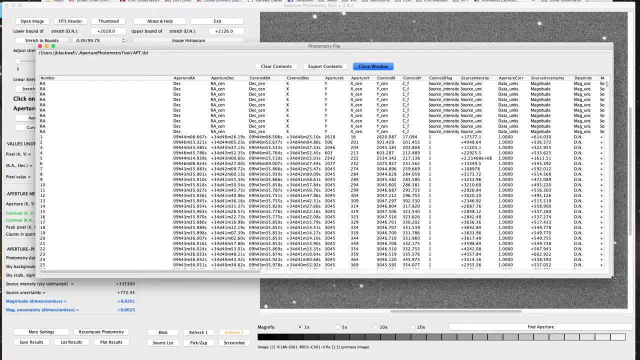 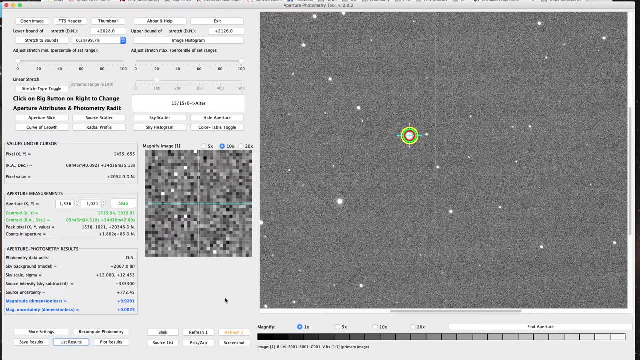 terms of the data And tell me that's not cool. It's all right there for you to play with. Okay, so that's what I have: How to set the zero point, Critical piece to understanding ABT, And feel free to email me if you have any questions or comments. We'll work on that. Thanks.